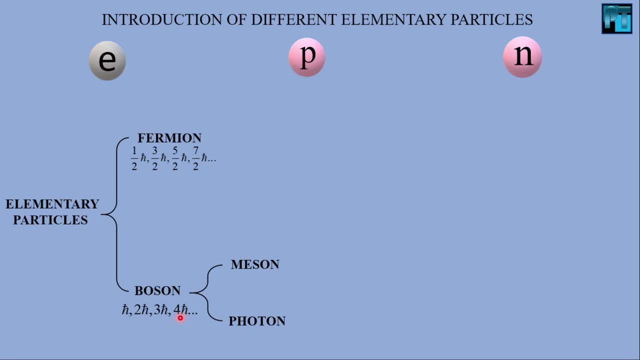 guys have already been introduced with photon. It is a very familiar particle, a quanta of energy. Now this meson category is further divided into three more categories, That is, pi-meson, k-meson and eta-meson. For the category pi-meson there are mainly three particles: pi-plus. 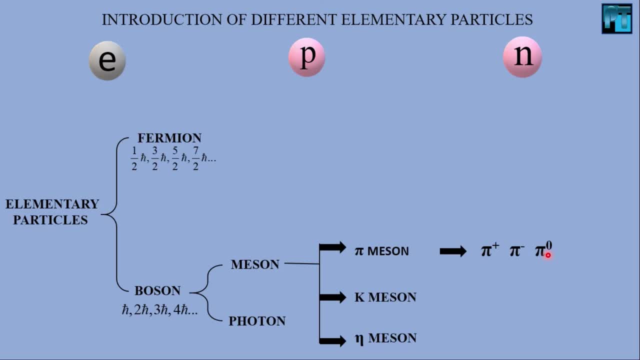 pi-minus and pi-zero. Similarly for k-meson there are two particles: k-plus and k-not. Sometimes these pi-mesons are called pions And these k-mesons are called kaons. In my total series I shall define this pi-meson. 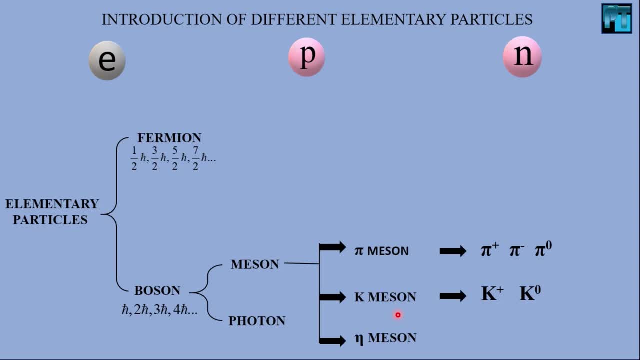 and k-meson as pions and kaons, So don't get confused in the latter And the remaining eta-meson In this category there is only one particle called eta-not, Now the fermions. Basically it is divided into two categories: eta-meson and eta-not. 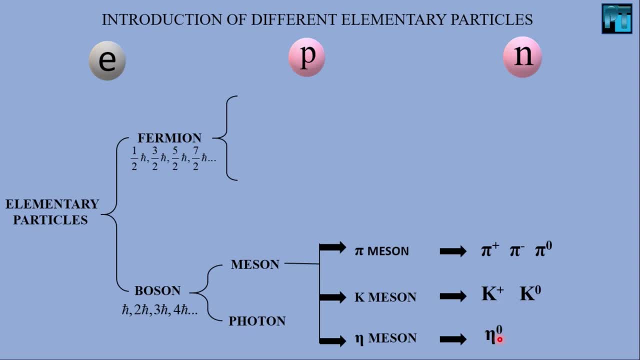 Now, in this category there is only one particle called eta-not Now the fermions. Basically it is divided into two categories. There are some of them and some of them are not. So is divided into two primary categories like lepton and baryon. In lepton category there are primarily 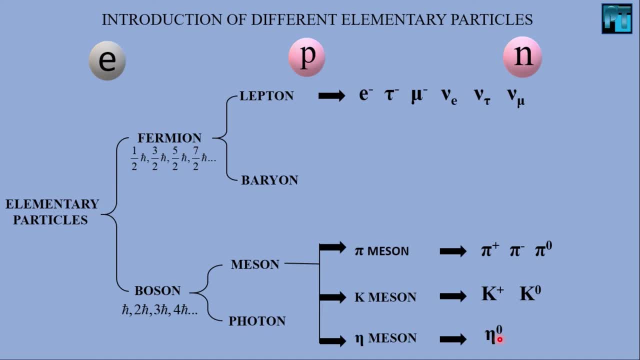 six particles or six type of particles: electron taon, muon and electron neutrino, taon neutrino, muon neutrino. These six particles mainly comprise the lepton family, Now the baryon family. Now this baryon family is further divided into two more parts. They are hyperon and nucleon. 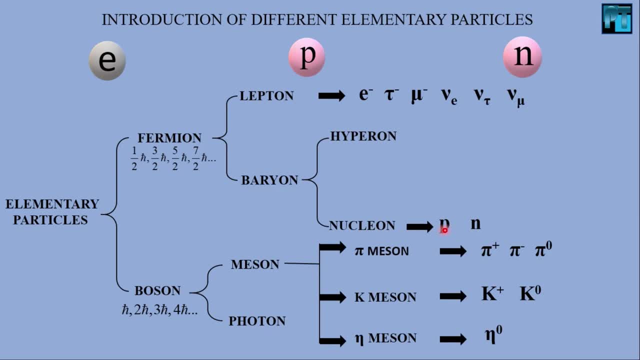 In nucleon family there is only two particles: this proton and this neutron. As you know that the nucleus is the nucleus of the nucleus and the nucleus of the nucleus is the nucleus of the nucleus, The nucleus of an atom is comprised of these two particles only. That's why they are called. 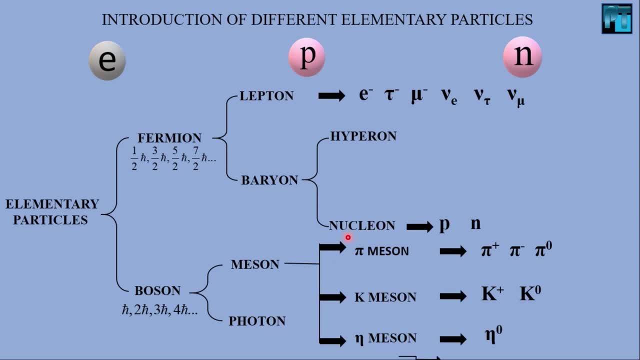 nucleons, Now the hyperons. There are further four categories in this type of particles. They are lambda hyperon, omega, hyperon xi, hyperon, sigma hyperon. In your textbooks sometimes it is called KSI hyperon, So whatever may be. Now, in lambda hyperon group there is only one particle called lambda naught. 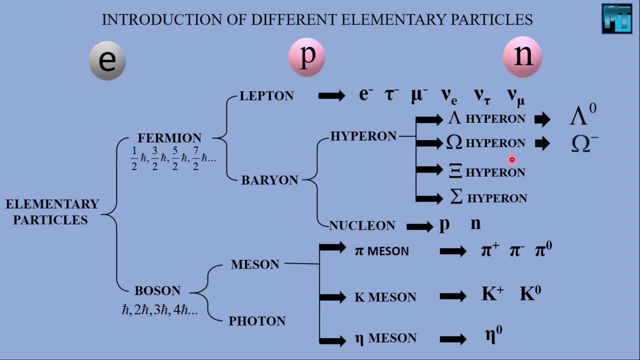 In omega hyperon family there is only one particle, omega minus. In xi hyperon family, there are two particles, xi naught and xi minus, And the last but not the least, the sigma hyperon family. It consists of three particles: Sigma plus, sigma naught and sigma minus. Now, this is a very simple structure of elementary particle. 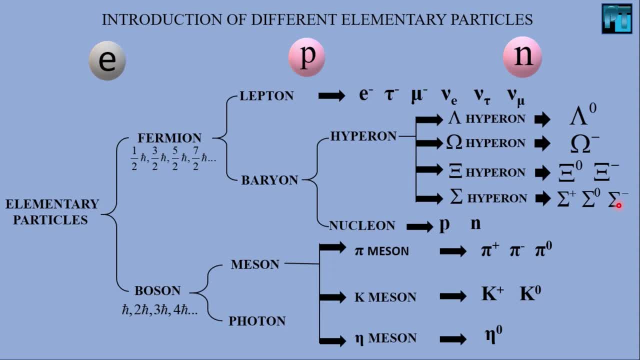 There are further, more and more particles like vector bosons, w plus minus bosons, z bosons, delta particles. There are more and more particles. Okay, but for the sake of simplicity, we shall discuss about only this family. I know that this picture is a little bit clumsy to you, but bear with me, guys, because this is the most. 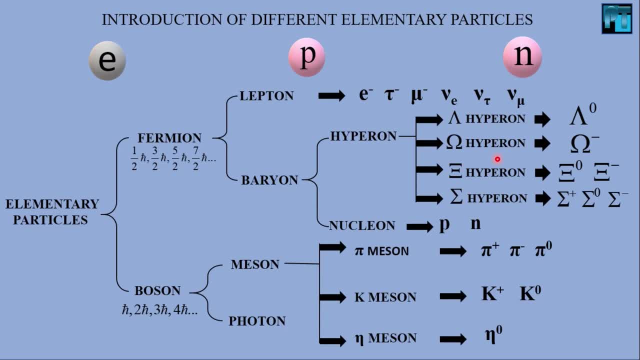 simplest structure I have. In your text books you can find other table type structures, but believe me, this is the most simple structure And you have to remember all of these particles. so this is your first task: to remember this structure, this family structure. now, these Kaons and these Hyperons are: 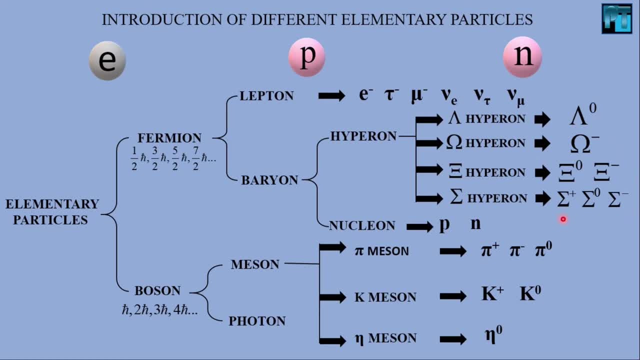 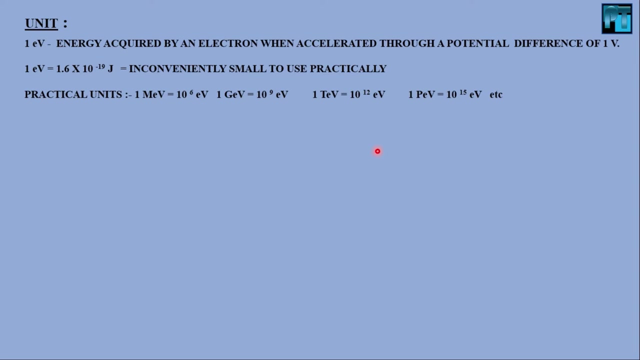 together called strange particles- the cause I shall discuss in this video later- and these pi mesons, k mesons and Hyperons. they are all together called hadrons. okay, now the unit. in this particle physics world we deal with energy units, mainly energy units like eV. what is an eV? one eV equals to the. 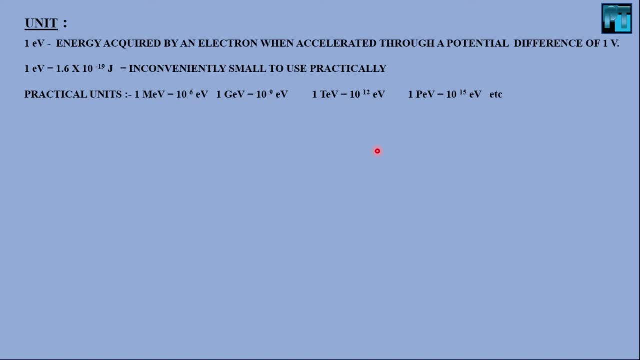 energy acquired by an electron. when it is, it passes through a space where there is a potential difference of one volt only. so one electron volt means one electronic charge. into one volt. there is 1.625 minus 19 joule, but this unit is inconveniently small for our practical usage. so what are the? 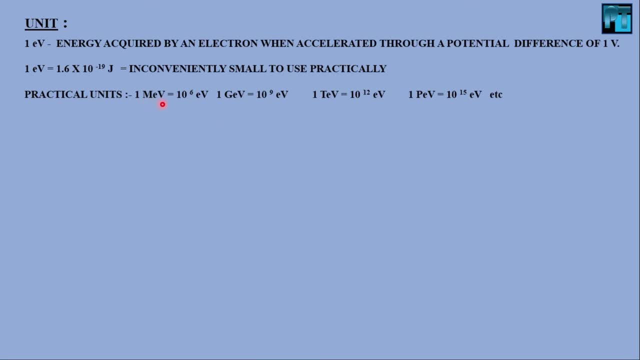 practical units, mainly this million or mega electron volts, giga electron volts, tera electron volt, peta electron volt and etc. etc. but for our practical usage and theoretical usage we shall start with this mega electron volt. okay now, as I have told you before that every unit we shall use will be in energy unit, 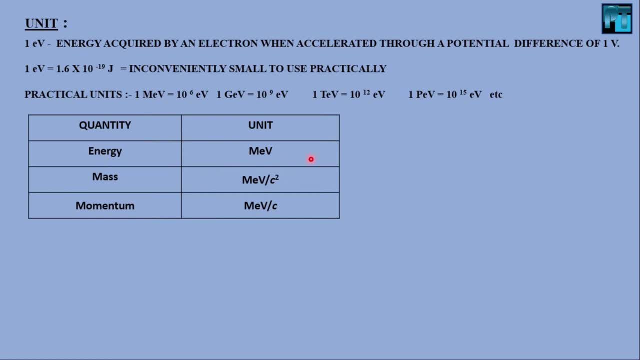 see, energy unit is MeV. so what will be the mass unit equal to mc2? so m equal to e by c square. what is the unit of e? that is MeV, and c square is c square. so mass will be defined by MeV per c square unit. in some cases we can take for simplicity: c equals to 1. okay, and for the momentum, 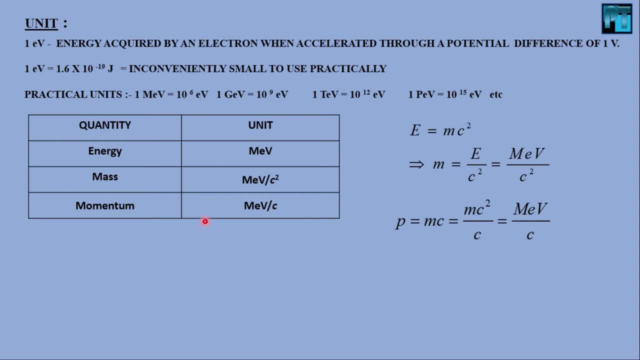 p equal to mc, mc squared by c, so it become MeV per c. so these three are the main units of our theoretical purpose. now there are some useful quantities, or say quantum numbers, and some formulas you have to know before entering in the particle world. what are those? 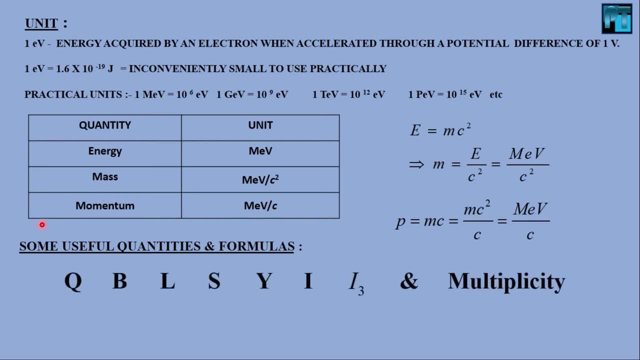 those are these quantities. you know, this is, this is a charge. B stands for baryon. quantum number L stands for lepton. quantum number S stands for strangeness. quantum number Y denote the hypercharge, I denote isospin. and what is I? 3 it is. 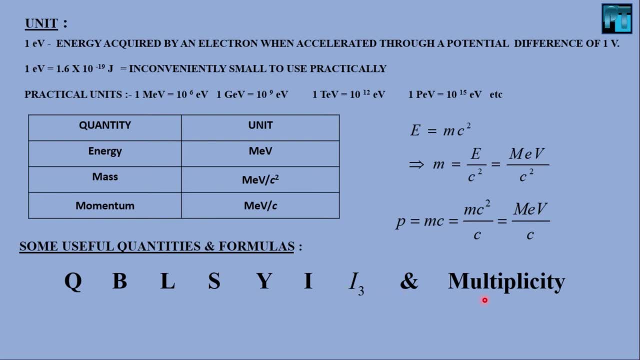 the third component of isospin and the multiplicity. actually, multiplicity is a mathematical term I shall discuss in this video. it is latter, and Y is equal to S plus B, Y is equal to 2 into Q minus I, 3. this thing is very, very important. 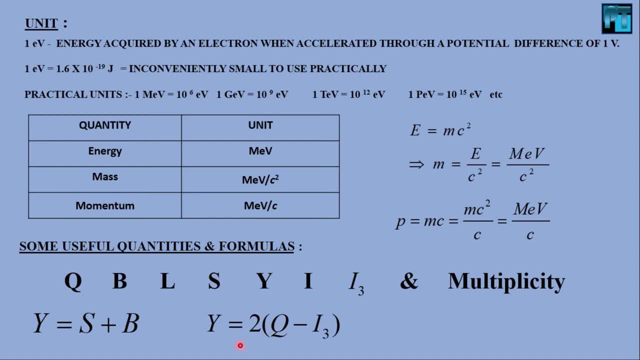 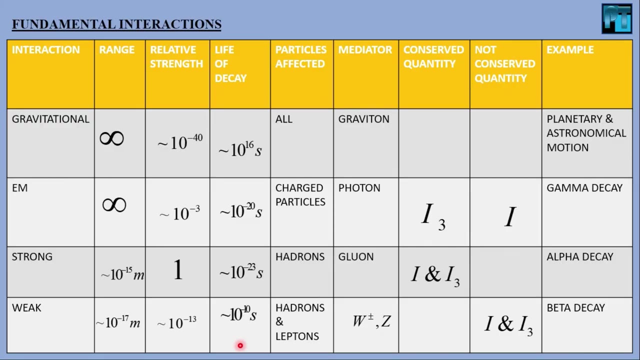 actually it is called Gelman-Nisijima formula. and the third one is a very known one: 2 I plus 1 equals to multiplicity. okay, now, this is a very important table for you. I have made these exclusive table for you because of: there are theories about these fundamental forces, but no proper. 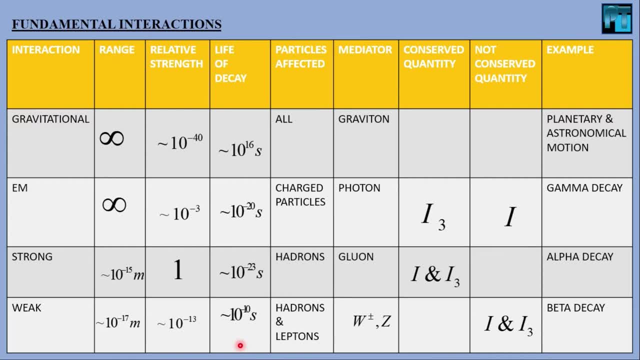 table for this. see, you can watch table for once. you will know that. okay, this is the main important parts and i have to remember these only so. in our nature there are four fundamental forces or, in technical word, interactions. what are they? gravitational, electromagnetic, strong and weak interactions between these four. in your 12th standard, you have already know about gravitational. 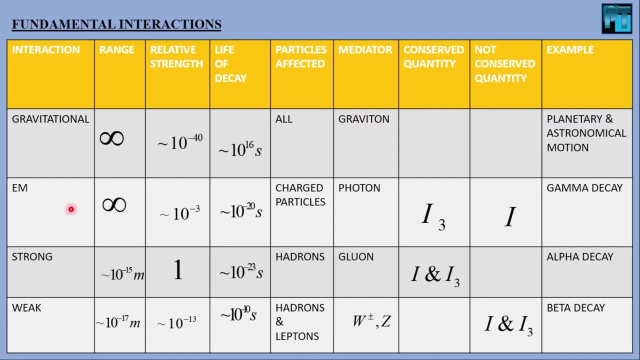 and electromagnetic. now in your graduation standard you will know about strong and weak interactions. now the first one is range. as we all know, by, theoretically these two forces are inverse square law. so as r tends to infinity, f tends to zero, so theoretically the range becomes infinity. that's why this range is infinity and strong forces are mainly. 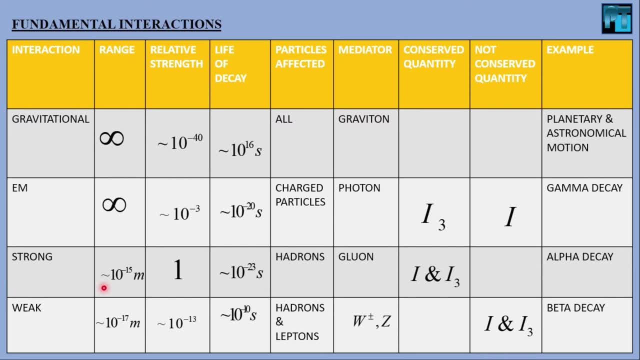 prevalent in nuclear structure type ranges. so it is more prominent in of the order of 10 to the power minus 15 meter type or fermi type range and weak interactions. they are the weak interactions have range of the order of 10 to the minus 17 meter. 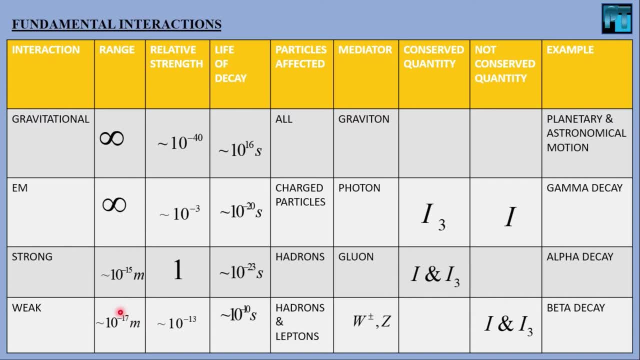 this is the single smallest strength. the point is it becomes limit then the most strong one, which is the poi. this is the most strong range between these four two- sorry between these four interactions, but according to relative strength value, it is very clear that strong interaction is actually very strong reaction interaction. that's why it's relative strength is one. this is the most strong intersection is one. it is the most strong interaction which we know in the video as it is something sub-inter Gardens. this is basредion, which means fast reaction. 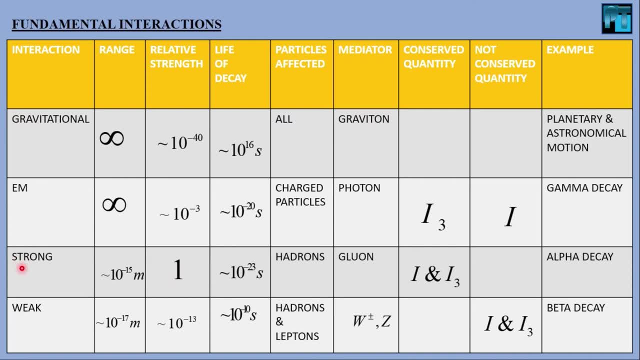 interaction. actually its name is wrong. okay, jokes apart, the weakest of these four interactions are gravitational interactions- see the number of the order: 10 to the power minus 40. then there comes the weak into the minus 13 and the electromagnetic into the minus 3.. 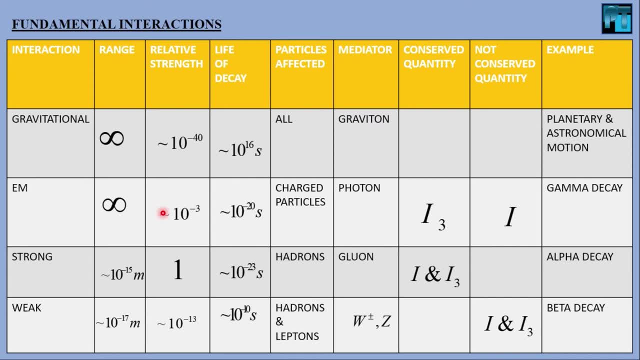 now life of decay. sometime it is called interaction time, sometime it is called characteristics time. actually it defines the actual interaction time of these four forces. in this table it is very clear that the time of interaction is highest in gravitational type fields. actually it is very common because gravitational force have an infinite range. 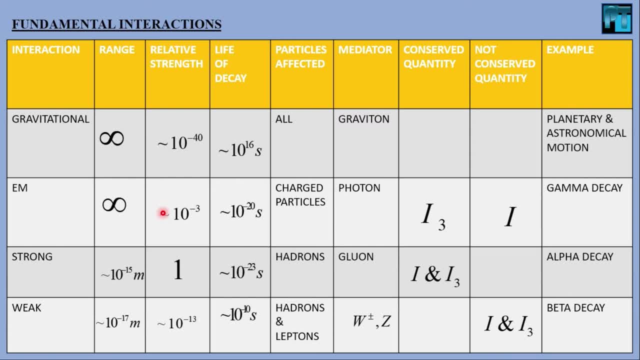 so the time of interaction must be the highest and time of interaction is the smallest in strong type of interactions. you now what particles gets affected by these interactions. actually, gravitational forces are not that much important in our particle physics or elementary particle physics chapter, because generally gravitational forces 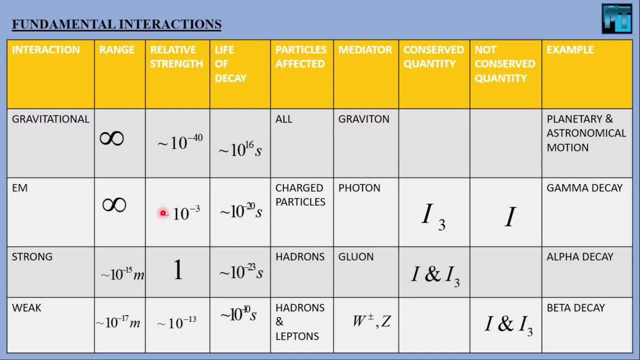 are prominent in astronomical entities or astronomical quantities like sun, moon. this type of macroscopic world gravitational force is prominent. but when the distance between two particles is very small or the particle itself is very small, like an atom or a subatomic particle, gravitational force is not that much important. 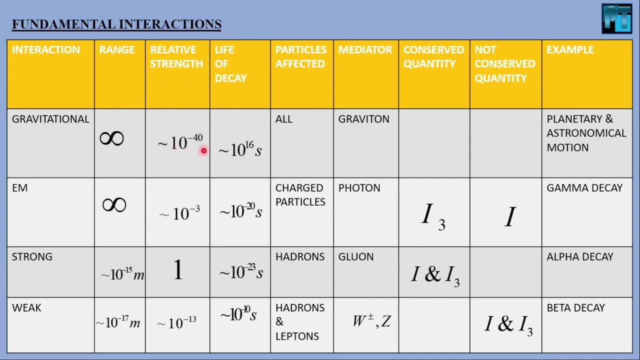 see the relative strength into 4 minus 5. it is important. so gravitational force is very important. T So it is not that much important and we shall not discuss about this force in this particle physics chapter Now from this table. it is very clear that gravitation affects. 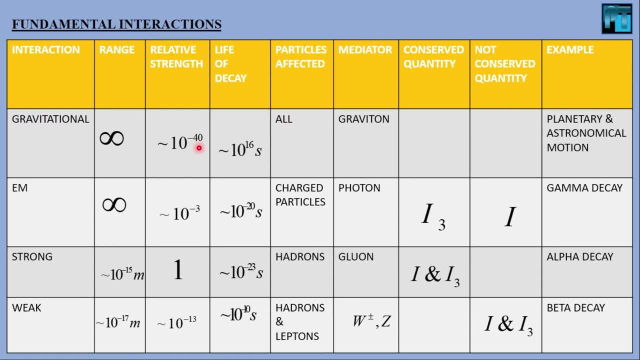 almost every particle in this universe. And what about electromagnetic? Its name suggests where there is a charge, electromagnetic field is there. So all type of charged particles are gets affected by electromagnetic force or interaction. What about the strong interaction Hadrons? What are they? I have already told you: pions, kaons and hyperons. These three. 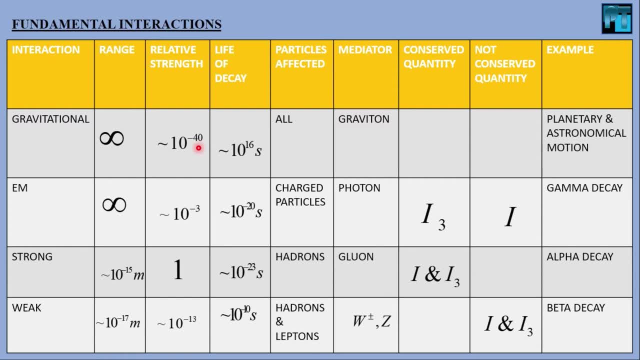 are called hadrons, So they take part in strong interaction. so they gets affected in the strong interaction. And what about weak interaction? Hadrons and leptons? Those six particles, taon, muon, electron and three types of neutrino- those are leptons and the hadrons. They gets affected in weak. 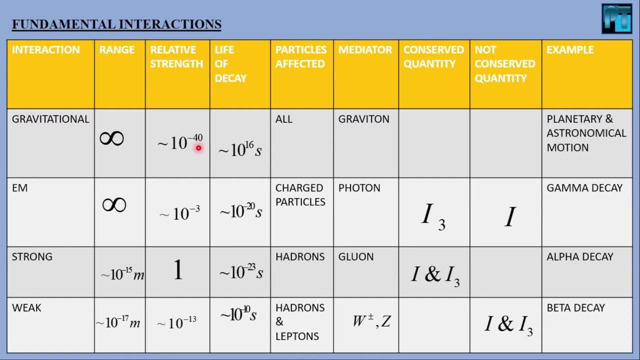 interaction Means they take part in weak interaction. Thank you and have a nice day. interactions now in this particle interactions or particle reactions, there is always a mediator particle or a exchange particle for gravitational interaction. it is called graviton. remember, graviton is still an hypothetical particle. no one have been discovered it yet, so you may be. 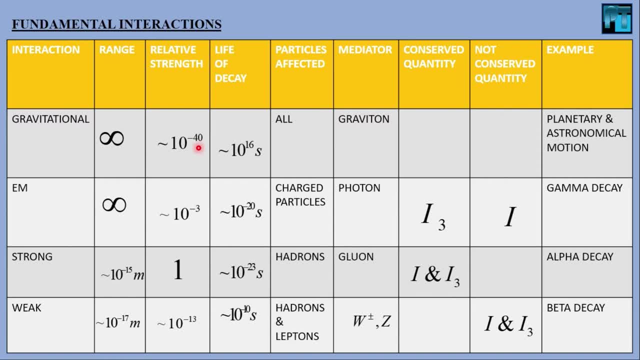 the luckiest person in the world who will discover the graviton and get the Nobel. now what about electromagnetic field? as only charged particles gets affected, its mediator or the exchange particle must be non-magnetic, none other than photon. what about strong and weak? now for strong interactions, see the hadrons takes. 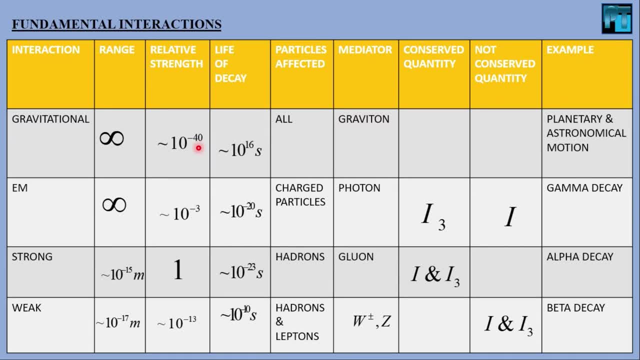 part and hadrons are made of quarks and theoretical as well as practical experiments have already shown that quarks have a mediator which is called gluon. so the mediator for strong interaction is gluon. in some of your textbooks you can find that the mediator for strong interaction strong 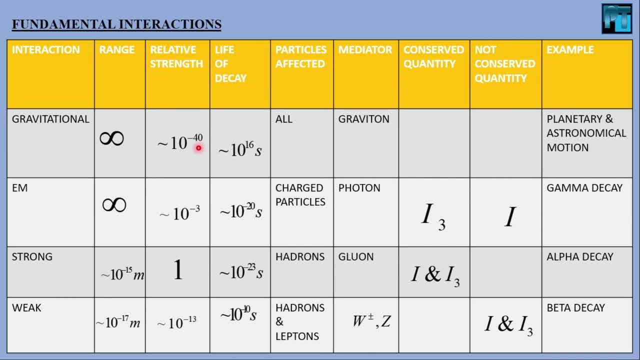 interaction is quark. that's also true. you can get the number of quark's interaction in your exam even more detail. gluon is the mediaton. now for the weak interactions. i have not shown these W plus, minus and z bosons in the previous family tree of elementary systems, Authority-Cathal. 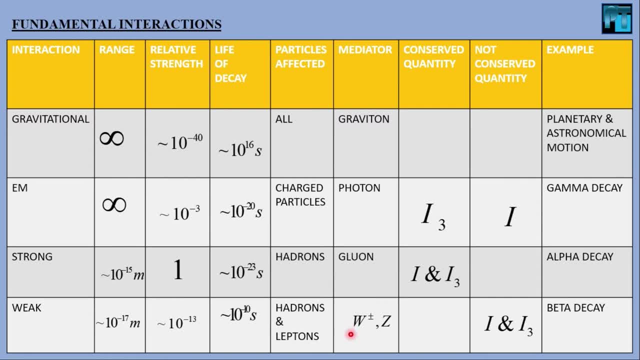 use this method, will click theấ� trying to create a routine using centimeters. alright, please enjoy the video. see you in the next video particles. these are relatively new and of greater importance than your BSc graduation syllabus, so I have excluded these exclusive particles in the 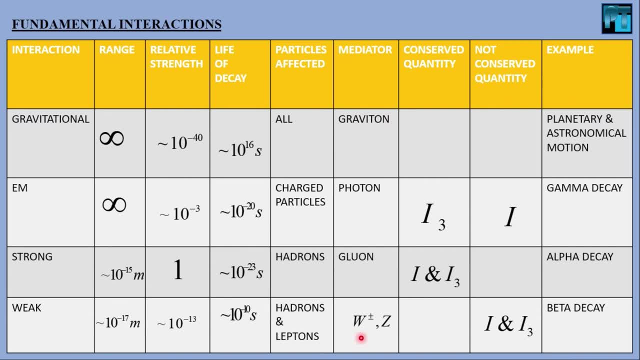 previous tree. only you have to know that the yes, there are some extra bosons, extra heavy bosons, like W plus minus boson and Z boson. these are not important for your graduation purpose. now, the most important two columns of this whole table: conserved quantity and not conserved quantity. now, see, I'm least. 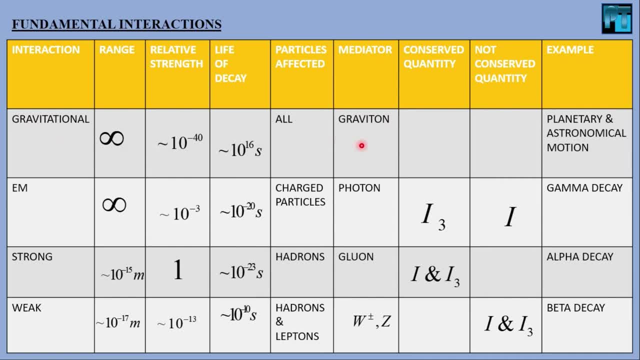 bothered about gravitational force in particle world. that's why I have left these two blank. and it's quite interesting that these two blanks are not conserved. quantity: and it's quite interesting that only i and i3 have been shown here. why? because there are several quantities, several quanta. 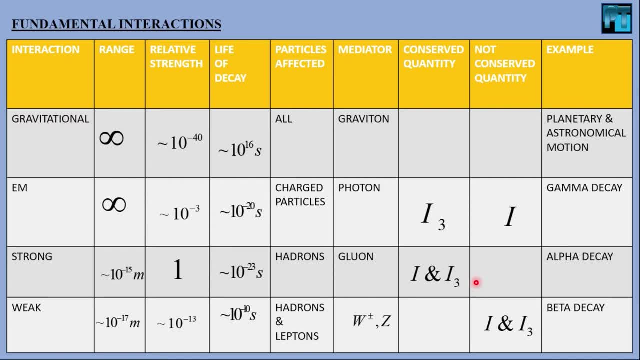 numbers, that some of them gets conserved in ea, more strong and weaker, some of them not like y, s, b, etc. etc. but we are primarily concerned about i and i3 because in your exam, as well as theoretical questions you have, you will have to determine whether 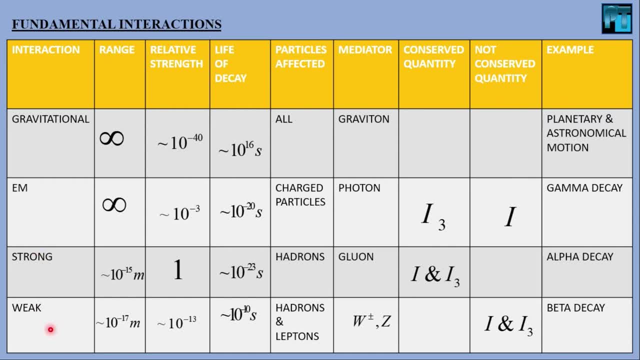 an interaction, is em strong or weak, and who will determine that this i and i3? if both of them gets conserved in any particle reaction, the reaction will be of strong type. if both of them will not be conserved in a particle reaction, then it will be of 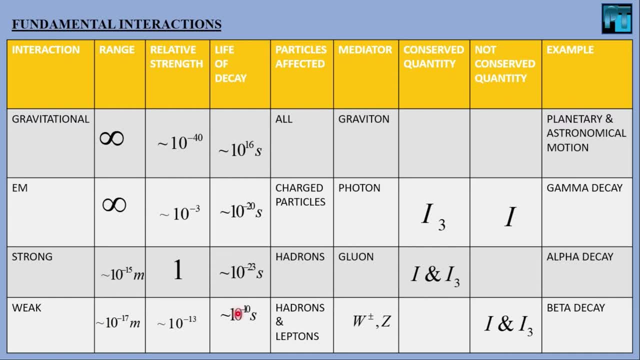 type weak. and if I3 is conserved but I not, then that is exclusively the electromagnetic interaction. so in your exam hall and your book there will be sufficient questions about: is this particle reaction possible? or say, determine the interaction about this particle reaction, then we will determine about the conservation of I and I3 and depending upon these three, 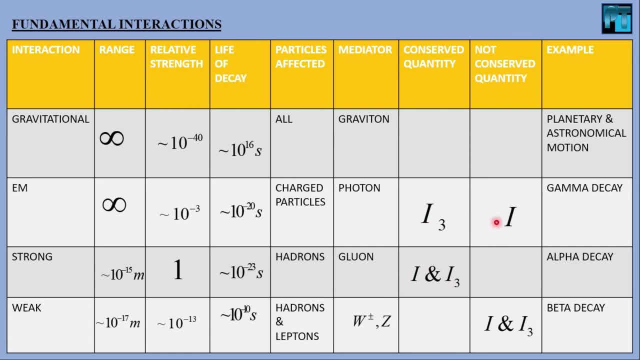 different, different situation. we can infer that, yes, that interaction proceeds through electromagnetic or strong or weak. I shall discuss about them in later lectures. and now that example. these are the most simple examples, only for your exam purpose. you can find many more examples in your any text books. so let's proceed. but before I proceed to more slides, 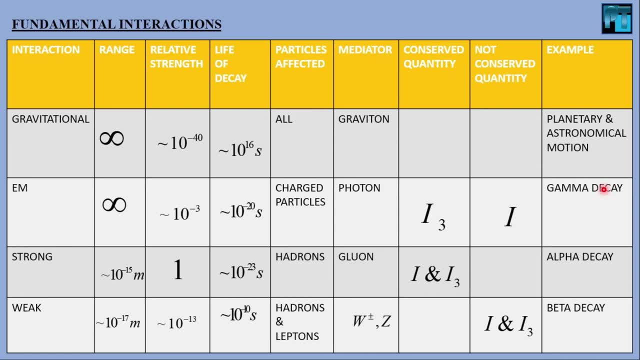 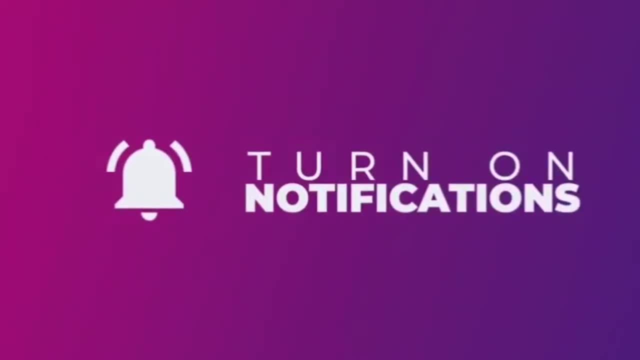 I have to remember you one thing: that if you are new to my channel, then don't forget to subscribe and click on the bell icon to get the regular updates, because this will be a series of, this will be a series of. this will be a series of. 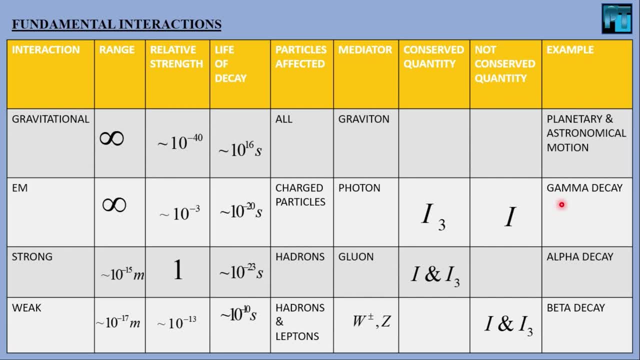 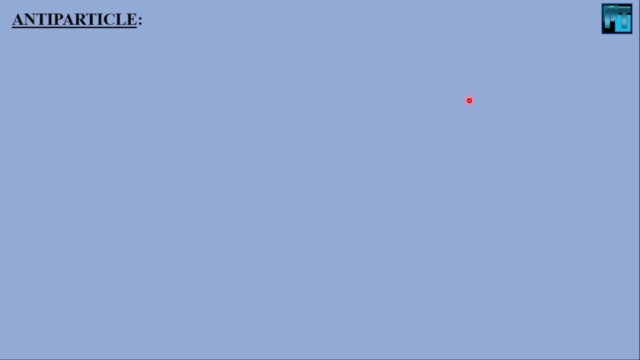 lectures, particle- sorry, elementary particle series. so to get the regular updates you have to be a regular subscriber. okay, okay, now let's proceed. now we shall discuss about antiparticles. before I further proceed about antiparticles, I have to tell you one thing: that particle physics is very much. 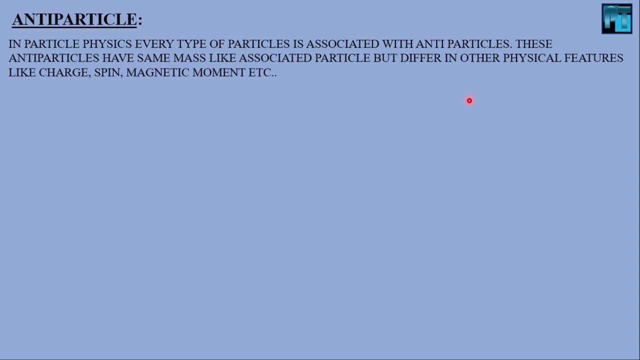 a theoretical field as well as practical field. why? because in earlier days, mathematically, some particles were inferred before their actual discovery, and after some years experimental physicists discover them in the practical particle accelerators, or particle accelerators or molecular mystery of the fa theta, you know things like exponential flow. 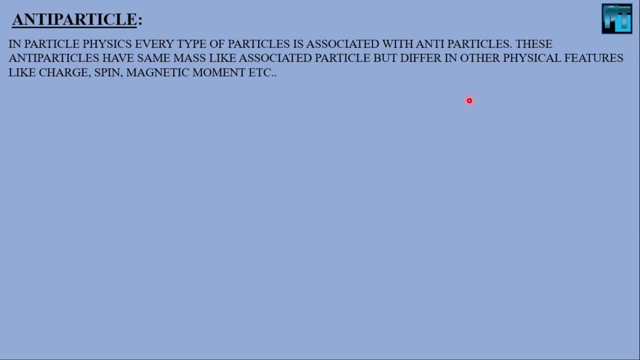 some other devices. an antiparticle is most important between all the theoretical concepts. see, in physics there is always a symmetry in natural laws. the mathematical symmetry shows that there should be a an't particle to each of the particles. in my first slide we have some family tree of particles. only I have not shown any type of antiparticles there. 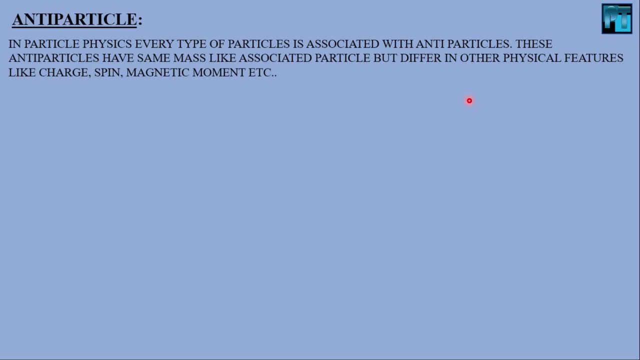 okay, though, every particle has an its own antiparticle, and these antiparticles have been theoretically inferred by some prominent scientists, and later they have been discovered in the laboratory. now you cannot find any antiparticle freely in nature. those antiparticles which will we, which we will discuss, are all created in lab conditions, and the most 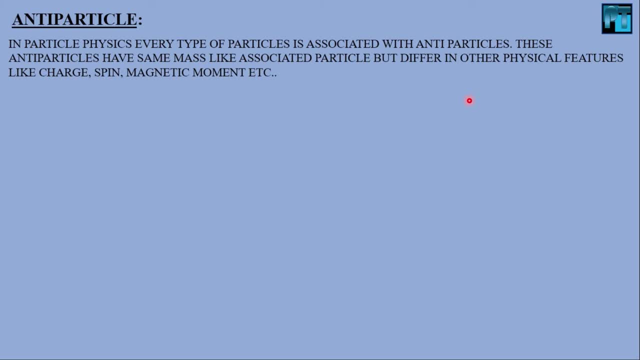 interesting part is that these antiparticles have mass, exactly the same about, about its antiparticle- sorry particle- but some physical features like charge and spin, trajectory, magnetic moment. they can be different, or actually in many cases they are exactly opposite to its particle counterpart, such as positron. 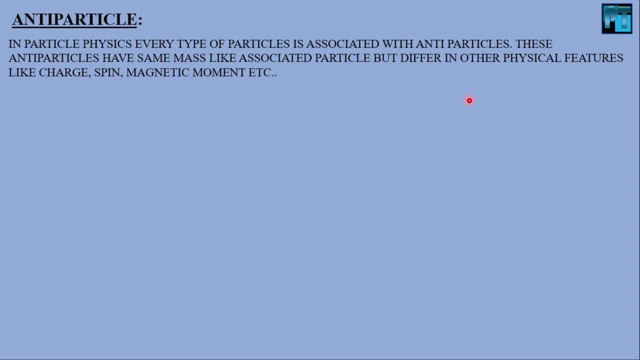 which has charged minus- sorry, plus one, and its counter particle is electron, which is which has charged minus one. actually, the first antiparticle discovered was positron. in, I think in 1930, Paul Dirac already predicted the antiparticle positron, and after two years, 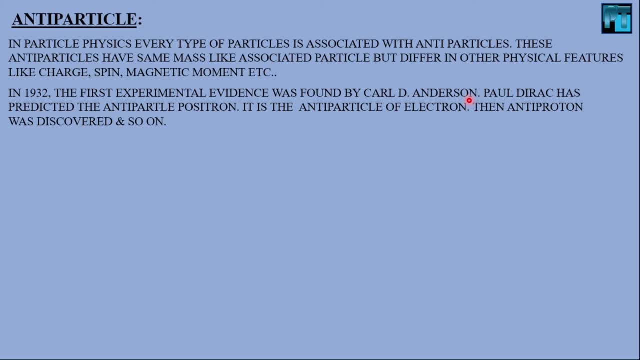 in 1932 Anderson showed the existence of antiparticle positron. this discovery of the positron is the evidence of existence of antiparticles for the first time. then, after two or three years, comes anti proton, then anti neutron, and then so on and so forth. 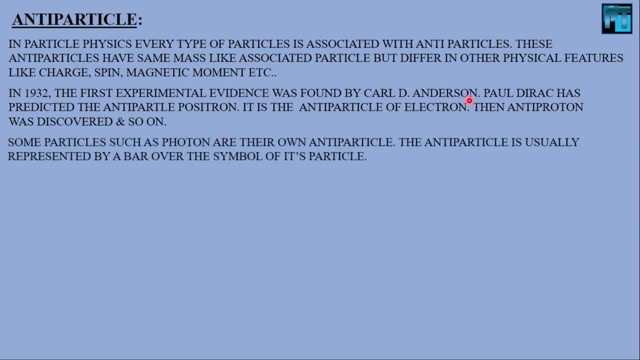 and then so on and so forth. now there are some particles also which are their own antiparticle, like photon, and we will denote these antiparticles like a bar over its head. okay, now I have already told you that anti particle is just an anti replica of your particle counterpart, as 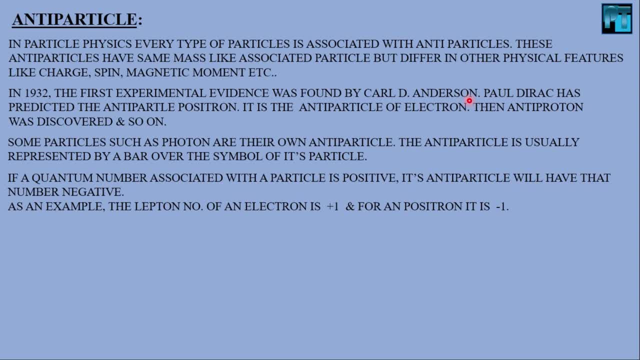 we denote every particle with some set of quantum numbers, numbers. so we shall have to denote these antiparticles with that set of quantum numbers, but the values will exactly the opposite. Suppose for an electron, if the lepton number is plus one, then for a positron it is minus one. This is the very interesting part about the 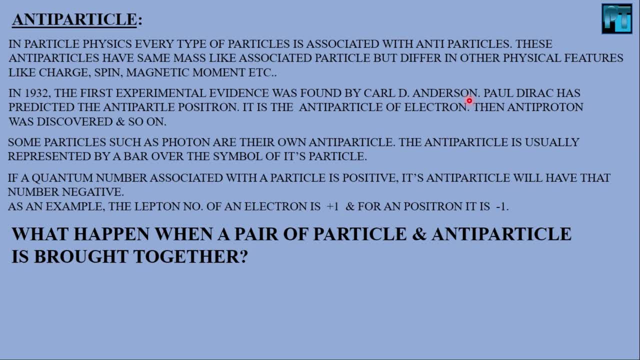 particle- antiparticle interactions. What will happen when a pair of particle and antiparticle is brought together? Suppose this is a particle, I have denoted it by x, and this is an antiparticle, I have denoted it with x, bar They are coming together. This is: 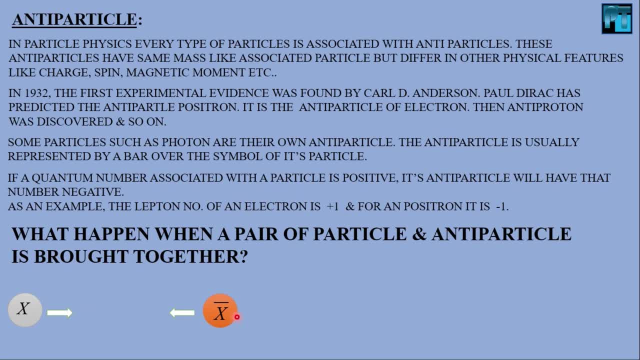 coming from this to this direction and this is coming from this to this direction. What will happen After some time? they will touch each other and what will be the result? Boom Means. they will annihilate each other and only energy will left. More technically, or 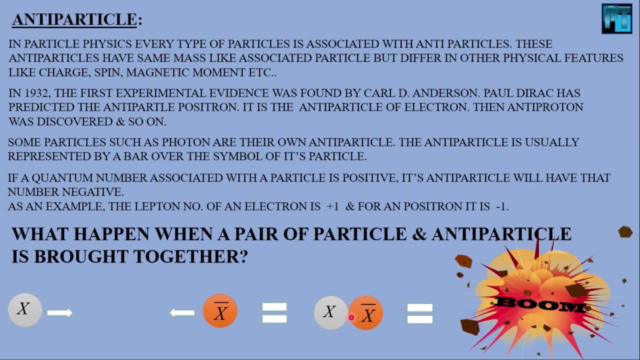 theoretically you can say, only photons will left. Okay, okay, I know that there is some questions, but still the biggest question: if a particle, antiparticle pair, can annihilate each other, then what will happen? Antiparticle pair can annihilate each other, So what will happen? 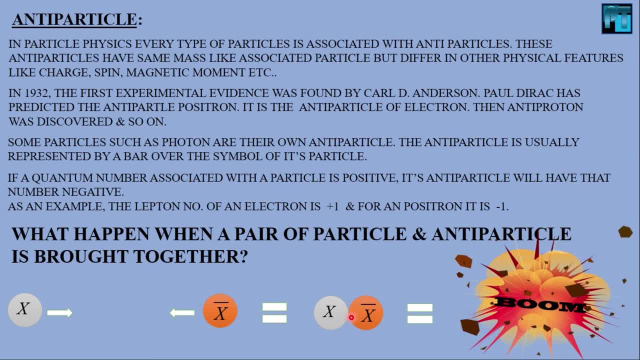 Now, if the particle- antiparticle pair can annihilate each other, then why do we exist? Big Bang says that there were exactly 50% of particles wereなので we exist. There is a big violation of these interactions. it wohl urine, the particle and antiparticle. 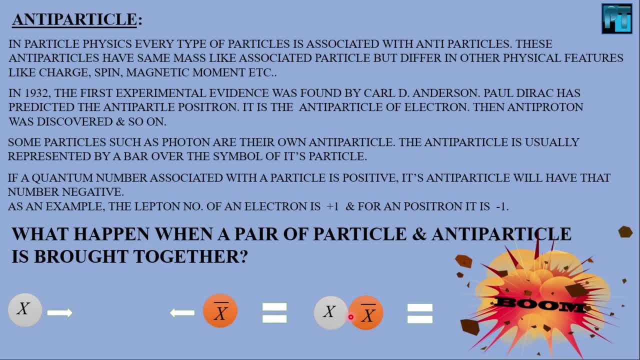 interactions. Some particles get annihilated by this problem. interactions and the matter. world dominates. now. theoretical scientists are doing their research to find the answer. let them do their job, and let me do my job: to teach you about the primary particle physics world. now let's proceed. 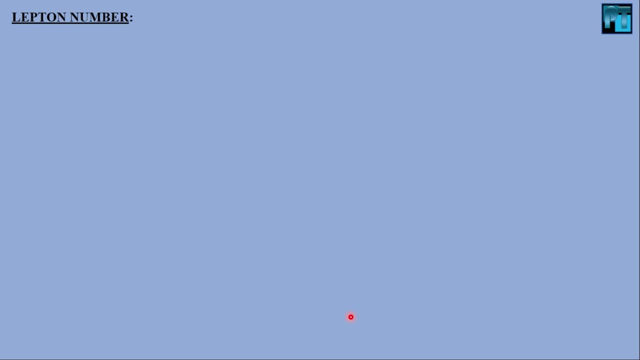 to next one lepton number. we shall denote lepton number by L. L is actually NL minus NL bar. what is NL, it is the number of leptons in a particle reaction, and what is NL bar, it is the number of anti leptons in that particular particle reaction. so it is very clear then that L is a number. 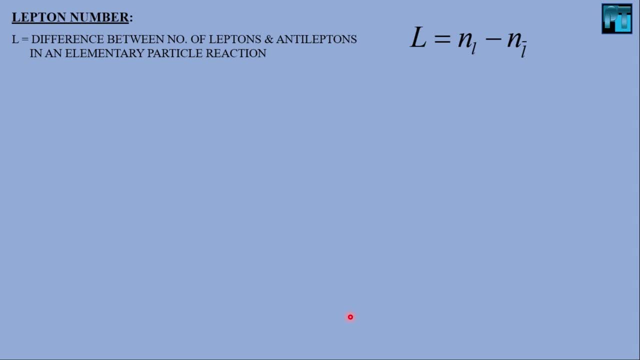 sometimes L is called lepton number, quantum number. actually it is a mathematical idea and it is. it is among some conserved quantum numbers. there are several conserved quantum numbers in particle physics world. lepton is one of them. now, in 1956, the famous Coven. 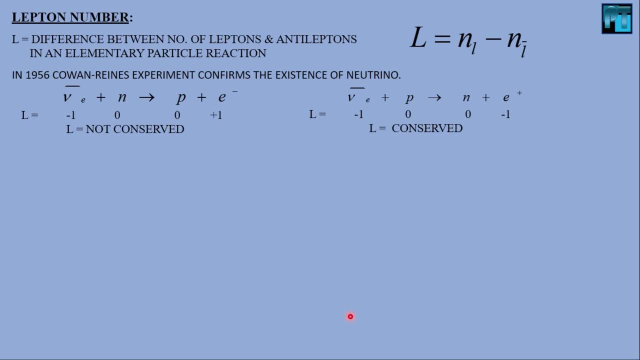 rings experiment confirms the existence of neutrino and this existence of neutrino. and this existence of neutrino and this existence of neutrino was inferred by L conservation theory. see, in this experiment, two type of reactions would have happened. there was 50-50 probability of this one and this 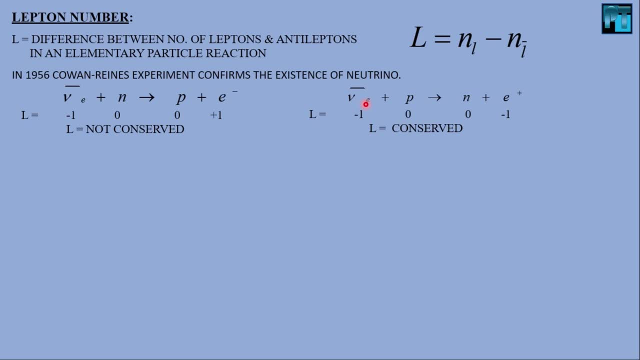 one. but in actual case, the experiment shows that this is the reaction that happened and this is the reaction that never happened. why L conservation theory longe to 0 is just 0? because it didn't object otherwise. L geçп약zuge is 0. this is Hanceyl pressure of the behavior of the 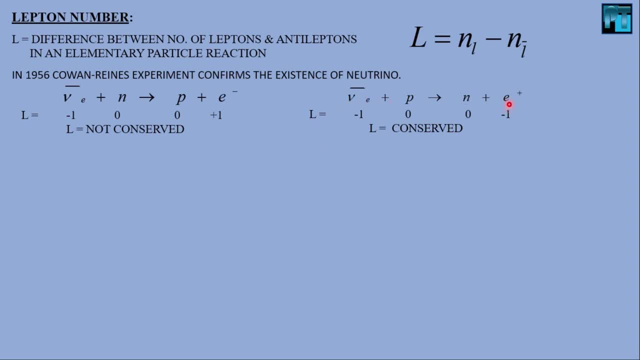 본. and then comes the idea of L conservation, because see, in this particle reaction lepton number is conserved. this is the entrance, it is at z-channel, and delta L equals to 0. so L is conserved, but in this reaction L is not. 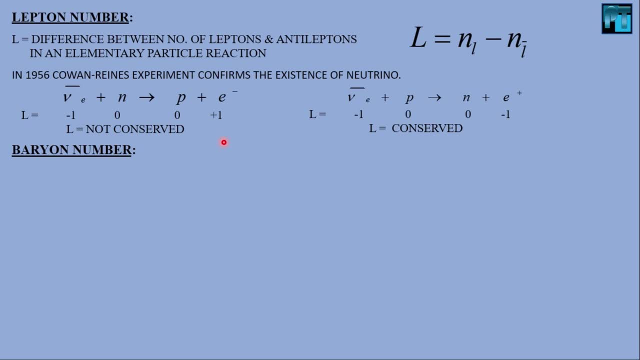 now, before i go to barrier number, i have to tell you one thing: that in your exam there will be questions like: will this particle interaction be feasible or possible or not? in that cases, we have to consider about some conserved quantum quantities. first of all, we have to see: 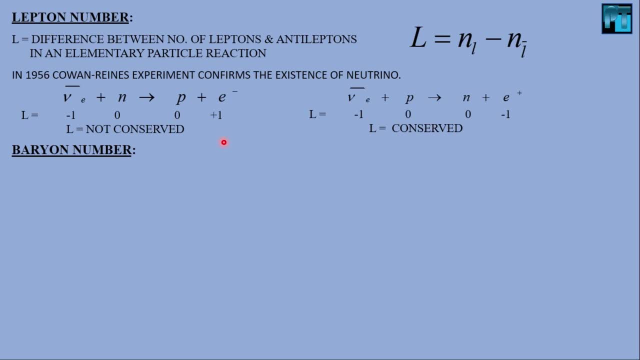 whether the charge is conserved or not, between the entrance and exit channels. if charge is not conserved, the reaction won't happen and thereafter we shall consider about some quantum numbers like l, b, s and etc. etc. depending upon the type of interactions or type of question. so 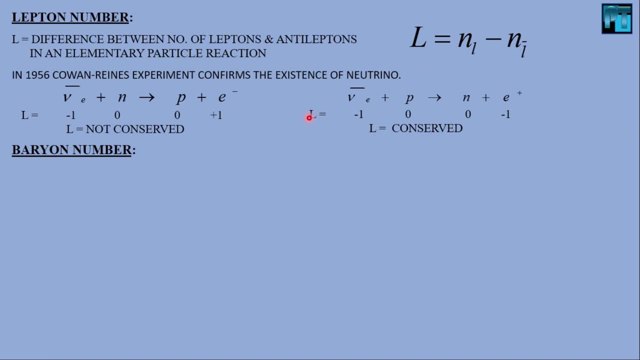 lepton number is very much important and by its name you have already know that lepton quanta number is important for lepton particles like that electron, taon, muon, electron, neutrino, taon, neutrino, muon, neutrino, this type of particles. so for them lepton number is plus one. see for electron it is plus one, but for 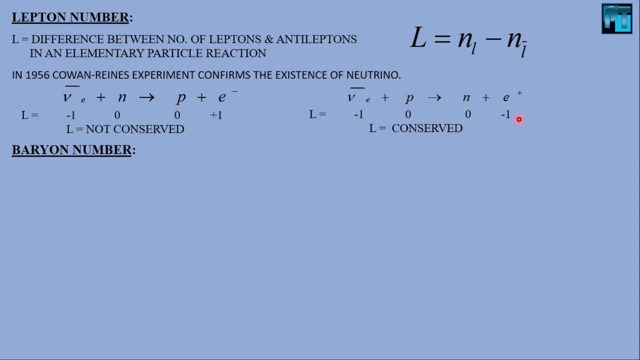 positron. it is minus one. so l equal to plus one for all lepton particles and l equal to minus one for all anti-leptons. see this electron neutrino bar. it is an anti-leptron. that's why minus one. now one more important concept: quantum number. that is baryon number it has. it is defined by b. 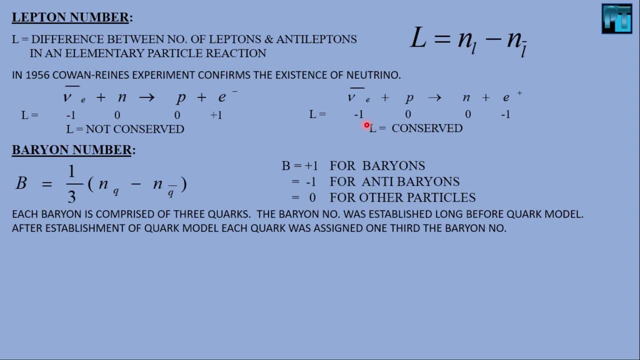 now, before i explain why this one by three comes, i have to tell you that baryon is not a computer number, it is just a Blafilm number. so there is no avoiding to the baryon number. baryon is a number set down at a transform inner convention. 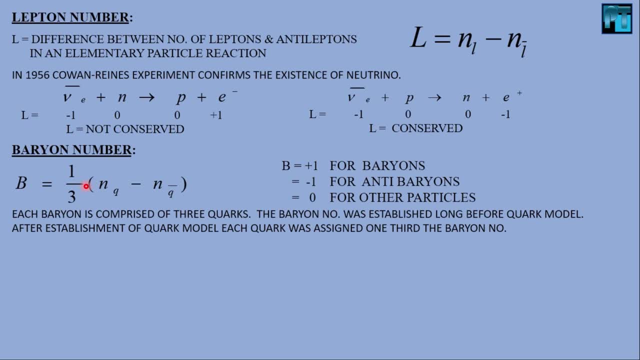 which is referring to an exceptionally interrupted test during which the spirits of a baryon part take place. they are mutated and constructed, and these are called quantum number, or what word we call baryon number, because we do not know how the name baryon's got related to the number. the very first variable is What Number. 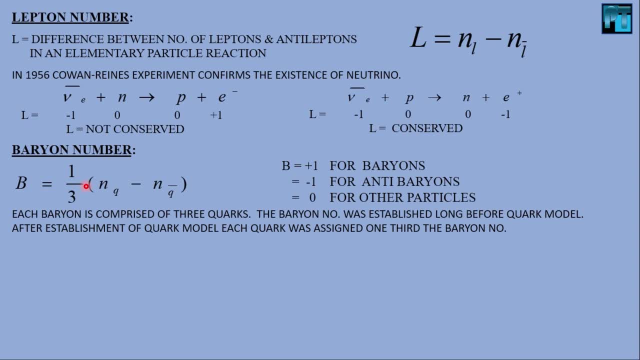 discovered. so scientists changes the baryon number of those quarks rather than changing the mother theory about baryon number. okay, so each quark was assigned by one third baryon number. why? because experiment shows that three quarks made one baryon, so each baryon is sorry. 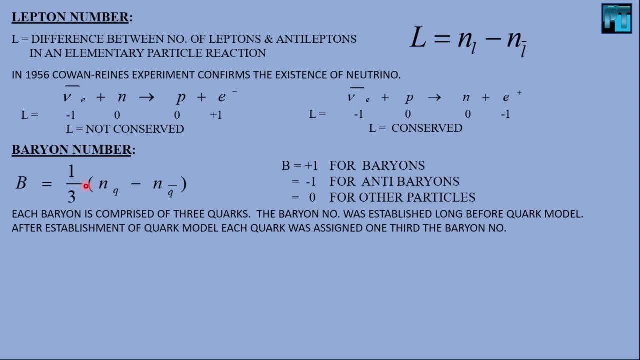 each baryon consists of three quarks. that's why each quark have baryon number equal to 1 by 3 and that's why this b, the definition of this b, has this: 1 over 3, nq minus nq bar. 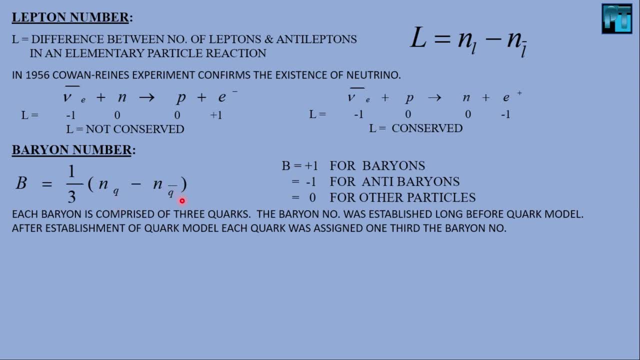 nq is the quark number and nq bar is the number of anti-quark in a particular reaction. now this b can have three values: plus one, obviously, for baryons, minus one, obviously, for anti-baryons. and what about zero for the rest of the particle world? 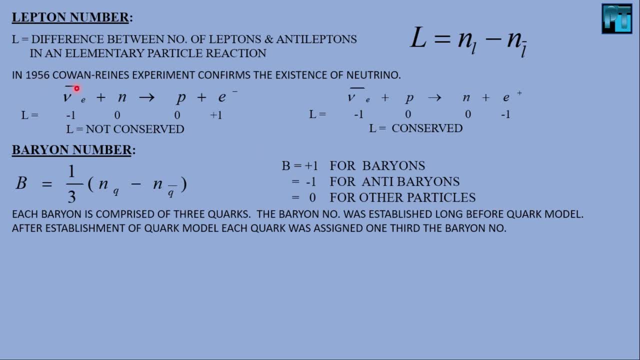 like for lepton. yeah, lepton b is zero. formation b is zero. now hypercharge: hypercharge is denoted by y. it is also a conserved quantity number, but for only strong interactions. in case of weak interaction, y does not conserve. y is defined by sum of s and b. but after the discovery, 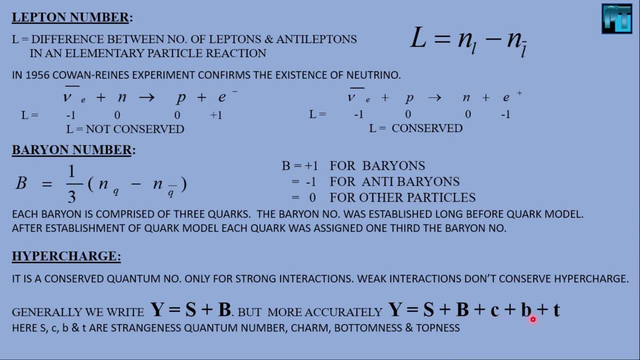 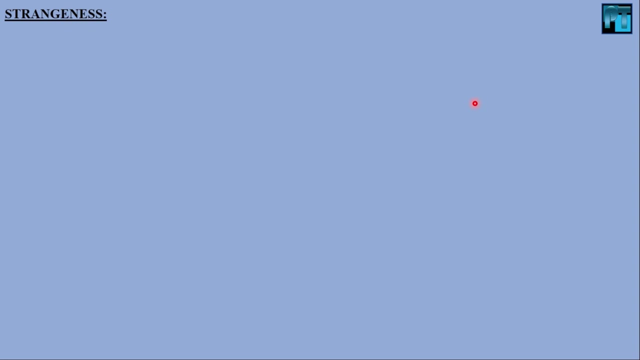 of beş u is defined as public change. I can compare it and you can write it as I can say these: Hi guys, awesome, not forget, you can subscribe my channel and I'll see you tomorrow. okay, bye. yes, it is another one of 4 preço yårcas. 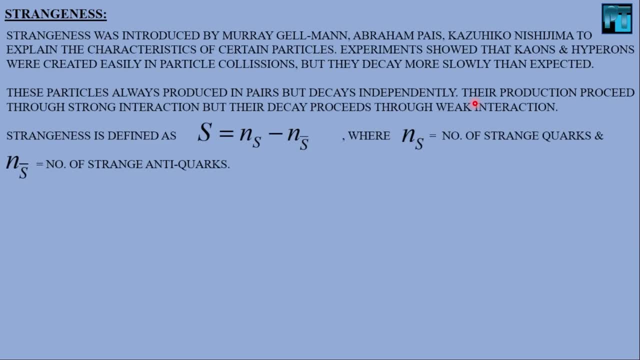 e. So strangeness is associated with a particular group of particles. that particles are called strange particles. I have already told you before that pions, kaons, sorry, sorry, sorry, sorry, very sorry, kaons and hyperons are collectively called strange particles. 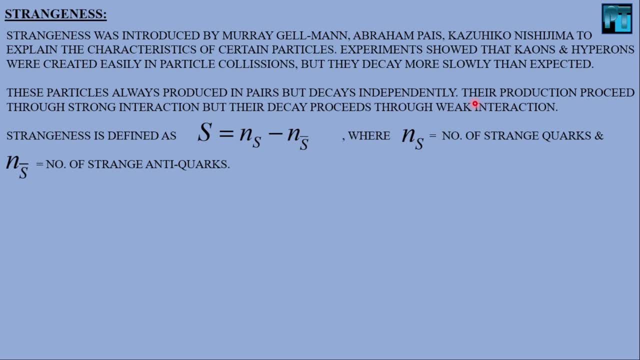 Why? Because there are certain characteristics which are unique, very unique. Experiments showed that these type of particles are created very easily in particle collisions, But they decay more slowly than theoretically expected. Moreover, these particles always produced in particles, But their decay process is very independent. They decay independently, Their production is called associative production and decay is individual decay. 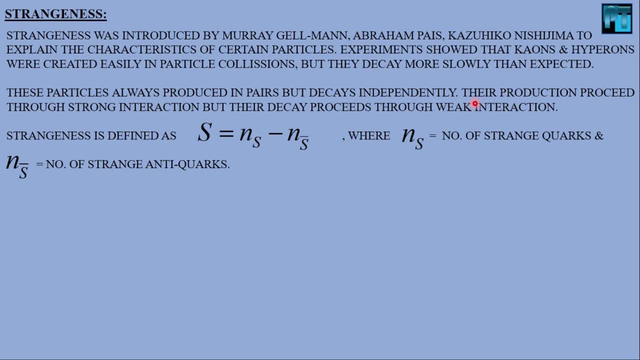 These two strange characteristics made them strange particles. Now strangeness is defined as s equal to n, So ns minus ns bar: ns is the number of strange quarks and ns bar is the number of strange anti-quarks. See, this is a very simple example of features of strange particles. 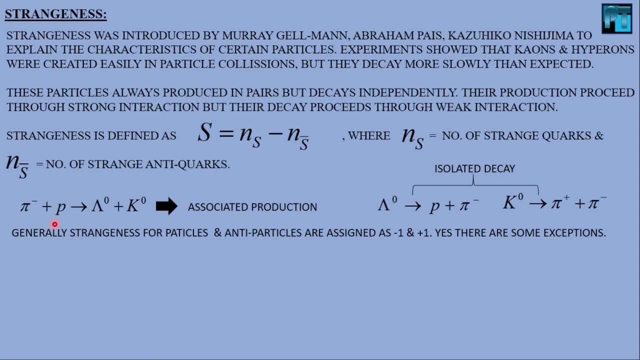 pi minus plus p. this reaction gives lambda naught and k naught. This is hyperon, this is kaon. So this is a associative production And these two strange particles have been produced in pair, But their decay process is entirely different. 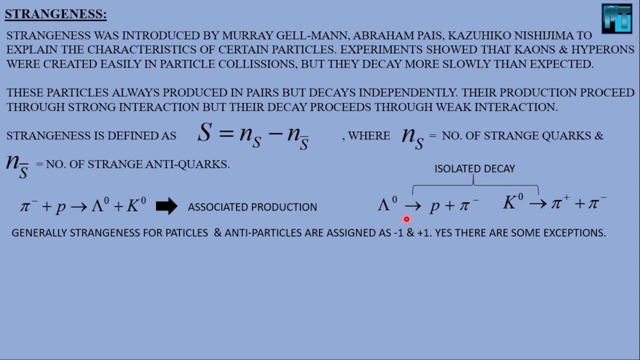 And the most interesting part is that they decay isolated. Like lambda naught decays into a one proton and pi minus, Whereas the k? naught meson decays into two pions. This makes them unique, and s is plus one for strange particles, or rather say particles, and minus one for anti-particles. 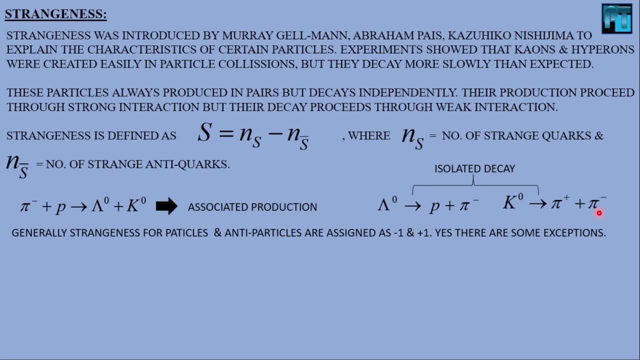 But there are some exceptions, like: s may be minus two, minus three, depending upon situations and for particular exclusive particles. that becomes true In my upcoming lectures. I shall show you the exceptions also Now. next, multiplicity. Actually, multiplicity is entirely a mathematical idea. 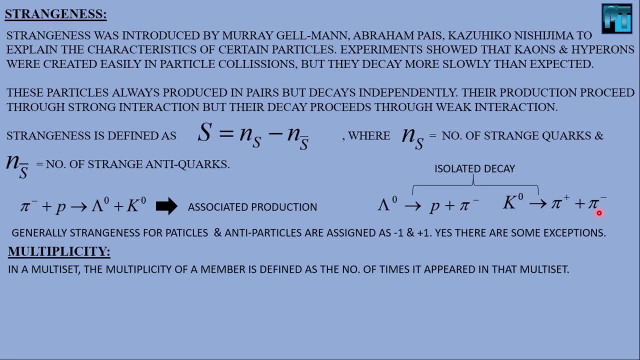 It is not related to only particle physics. It is related to multi-set type of mathematics. In very simple language, multiplicity is the number which defines that a particular quantity is repeated by how many times. Suppose, forty-five equals to what Five into three into three. 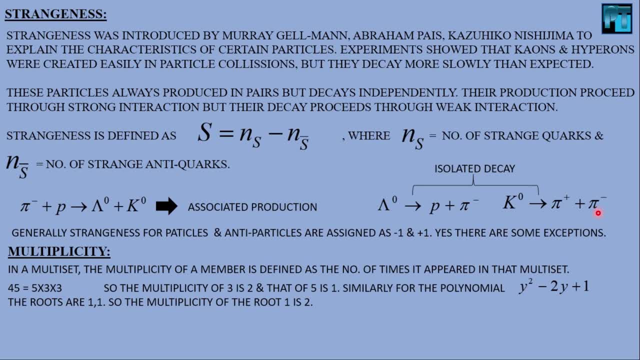 Actually five into nine. So I can divide nine by two, threes. Look, this three is repeating itself twice. So the multiplicity of three is two And multiplicity of five is one. This is the most simple example. 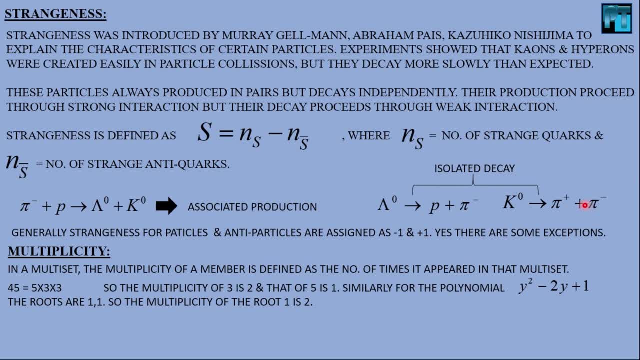 Now let us do some maths. This is a very simple polynomial: y square equals minus two, y plus one. Okay, What are the roots? Actually, it is y minus one whole square, That is y minus one. into y minus one. 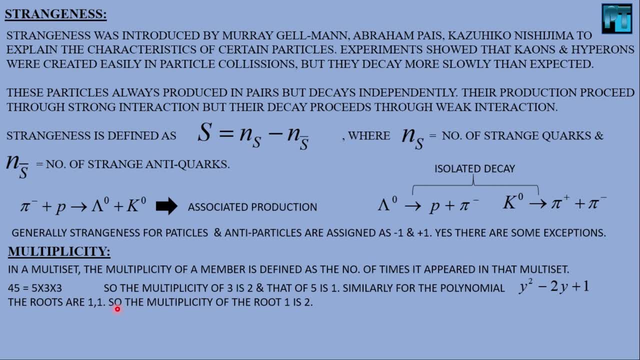 That is two roots, One one, So the root one is repeating itself twice. So what is the multiplicity of that root Two? Suppose we have a quantum number, Say that is x, Then what is the mathematical form of multiplicity? 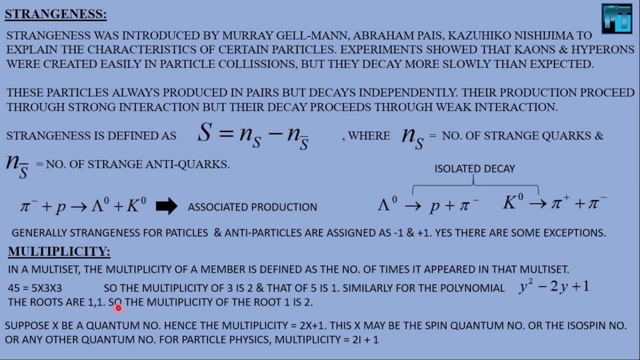 Two x plus one. I have previously showed you that multiplicity two y plus one is equal to multiplicity. Actually, in particle physics world we use multiplicity equal to two y plus one. y is the isospin quantum number. If we know the y, or if we know the multiplicity, we can define the other quantity. 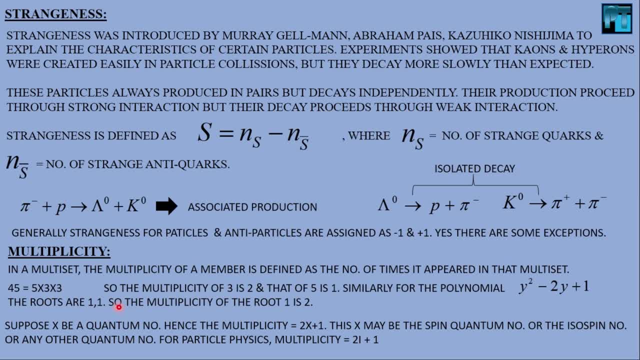 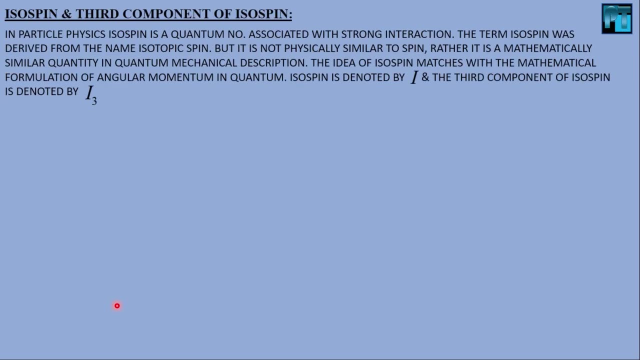 Suppose for pions. what is the multiplicity Three? So two. y plus one is equal to three, So y is equal to one, Depending upon the value of y. y three will change Isospin. Before proceeding I want to remember you that isospin and that y three that was called third component of isospin. 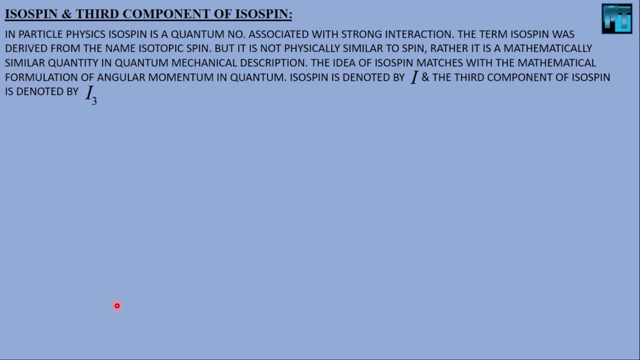 These two are very important for particle reactions as they determine the interaction type, whether it is electromagnetic or strong or weak. So in any particle reactions you have to determine whether i and i three are conserved or not. And to determine the conservation of i and i three you must know the values of i and i three of those particles. 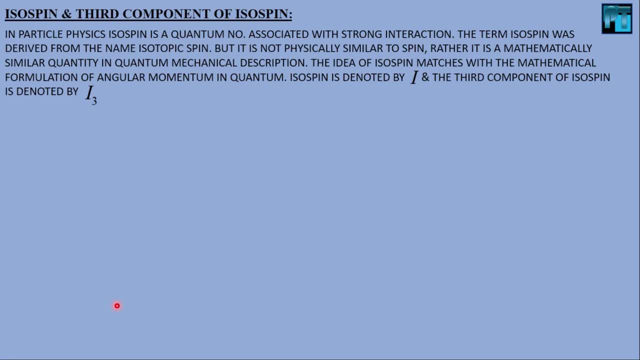 So i and i three are very much important for you, not only for your knowledge, but for your exams also. Now, the term isospin: though it has a term spin, it is not actually spin. It is a basic mathematical idea which has some similarity to spin. 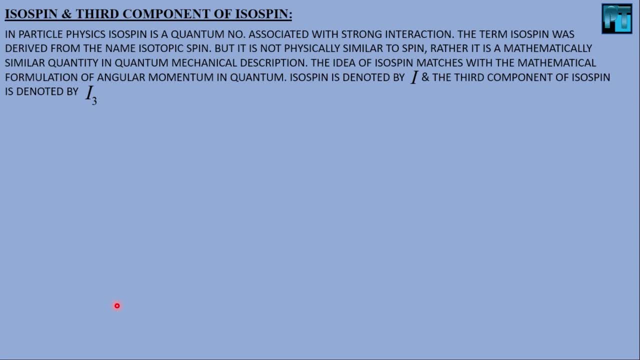 Rather I say similarity to angular quantum number. This isospin quantum number behaves like mathematical definitions of spin, but it is not physically a spin. Generally, isospin comes from the word isotopic spin, But isotopic spin is not the actual word. 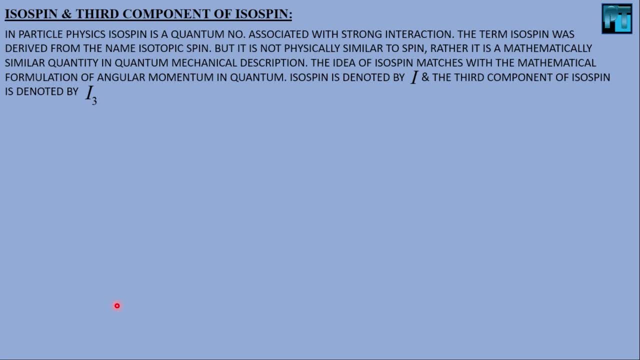 Physicists say it isobaric spin And i three is its third component. What is third component? Suppose you have a three-dimensional vector. What are the three components? The x, the y and the z. The z component is called third component. 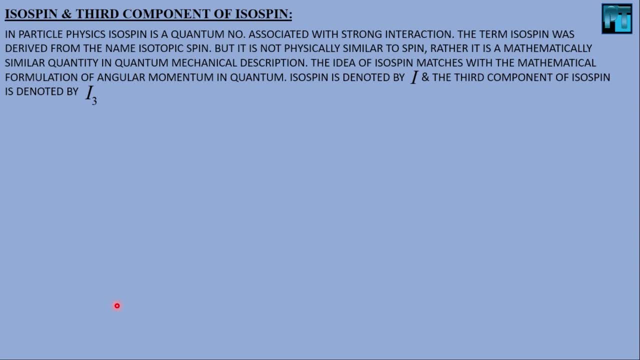 I can define one, two, three. one is for x, two for y, three for z. So i three is actually the z projection of i. Now I am giving you the information that i three is the z component. So who has z component? 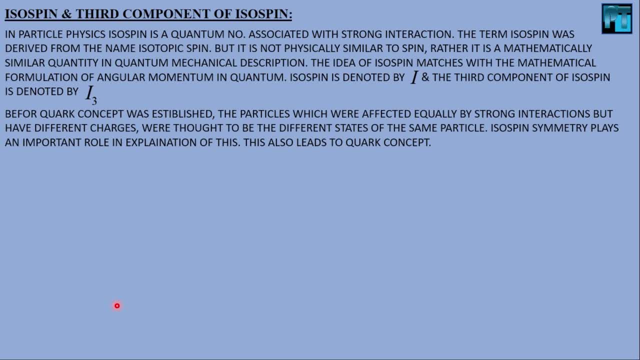 A vector- Actually i is- sometimes behaves like a vectorial quantity. This concept of i also supports the concept of quark model. I have not discussed it yet. In my coming lectures I shall discuss about that quark model. But before quark model there was i. 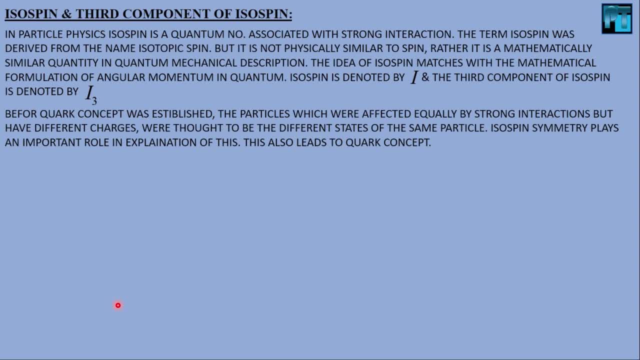 Why? Because experimental scientists find out that there are some particles which were affected in strong interactions equally, But they have different charges. So they thought that those particles are the same state of same particle. Suppose there are three charges, They thought that the mother particle is one. 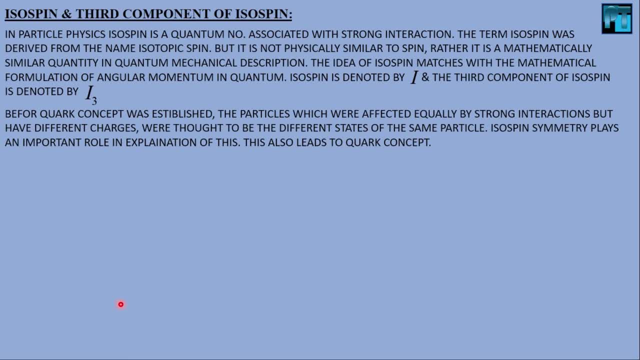 It is the three different states of that mother particle. Iso spin symmetry supports that fact, Or Iso spin symmetry is the mathematical formulation of that fact, And that fact in latter leads to the quark concept. Now the third component of i. 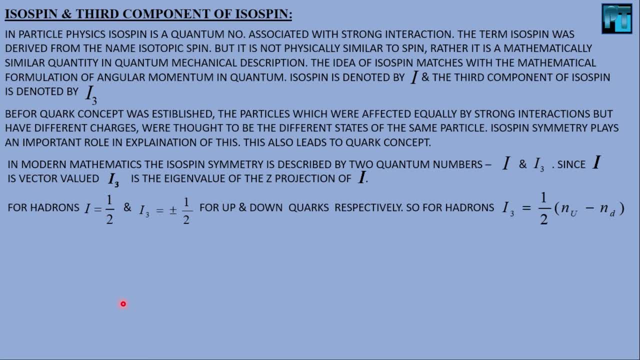 Now, before I proceed to that one, in some mathematical idea isospin is a vectorial identity, So it has three projections And the most important projection is z component. Actually the isospin quantum number comprised of two quantum numbers, i and i, three. 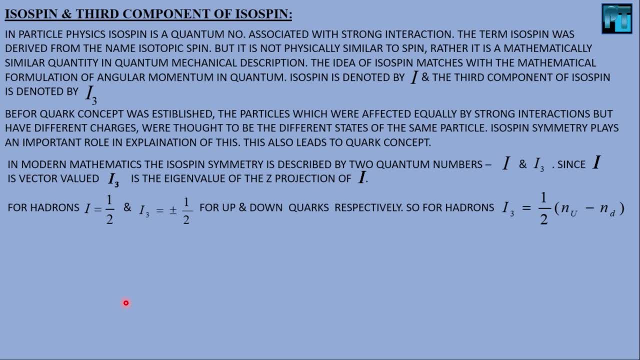 First you have to determine the i, Then the i, three. Now how to determine that 2i plus one equal to multiplicity. If you know the multiplicity, you can define. i like pions, i equals to one. 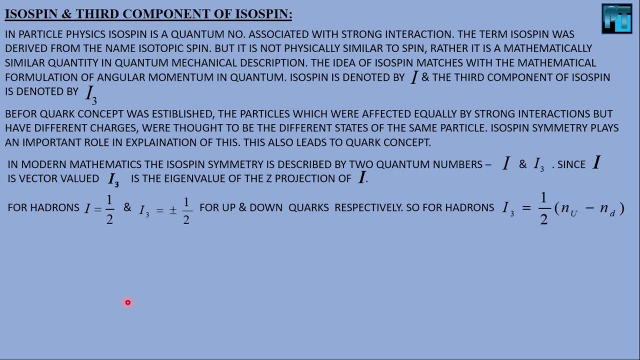 Now for hadrons or spin half particles. we have what We have: i equals to half. How See, in that type of particles, 2i plus one equals to two. So we have: i equals to half. If i equals to half, its z component can align itself to either plus half or minus half. 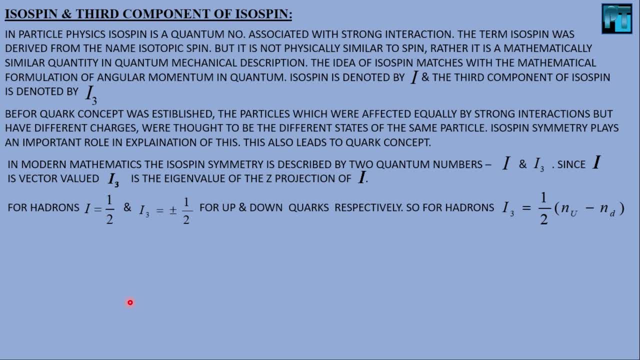 Plus half is associated with up quark and minus half is associated with down quark. So in case of hadrons we can define i three as half of nu minus nd. nu is number of up quarks in a particle reaction and nd is number of down quarks in that particle reaction. 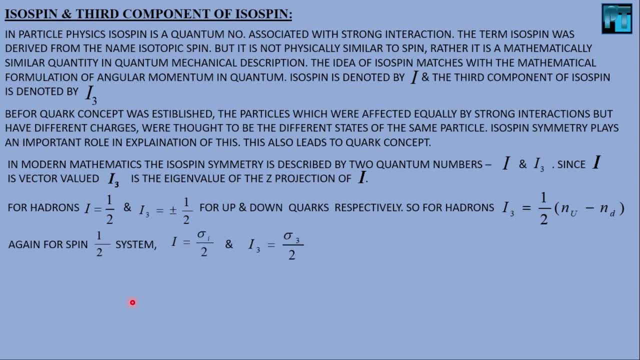 Now, this is for spin half particles. What about- sorry, it was for hadrons. What about for spin half system? Now, for spin half system: i is sigma i by two. What is sigma i? Sigma i is Pauli matrices. 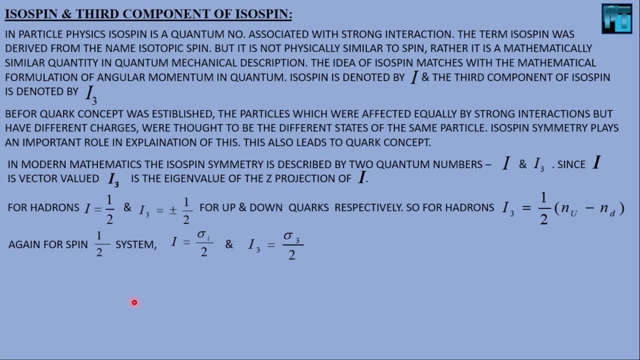 In atomic physics and, of course, in quantum mechanics, there are three separate matrices, two by two matrices- They are called Pauli matrices, And i three is equal to sigma three by two. Now in this lecture I have not shown what about sigma one and i three. 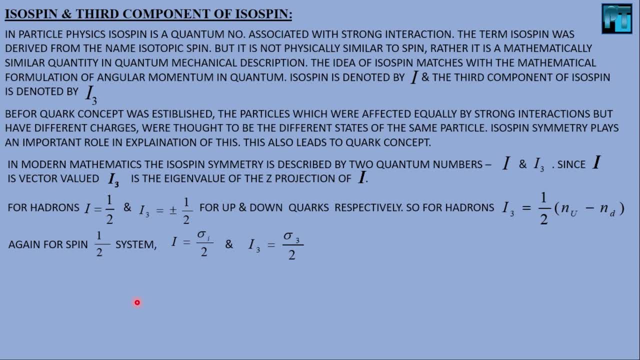 What about sigma one, sigma two, sigma three? What are their values? What are their characteristics? Because it is not important in here. If I have time, then in my later lectures I shall try to show you about that. Pauli matrices. 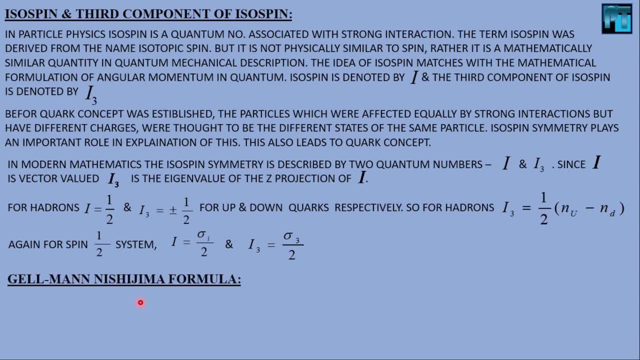 But it is not relevant in my introduction lecture. Now let's come to a very important formula, Gelman-Nisijima formula. You have already familiar with the Gelman-Nisijima formula, But the original formula was like q, equal to i, three plus half of s plus b. 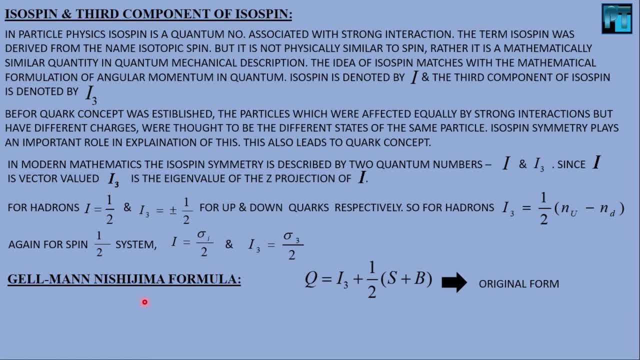 It was the original Gelman-Nisijima formula. Then, after the quark model, there comes three more quark numbers, or say quark quantum numbers. Or in some of your texts there are quark flavors. What are they? 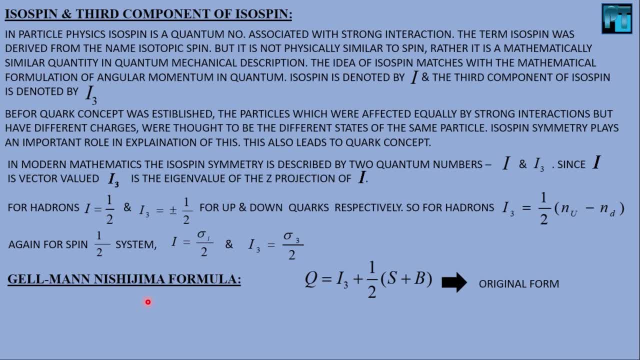 They are called bottom and top, c, b, t. So the more modern form is: q is equal to i, three plus half of s plus b plus c plus b plus t. Now, if we can put this s plus b plus c plus t with y, 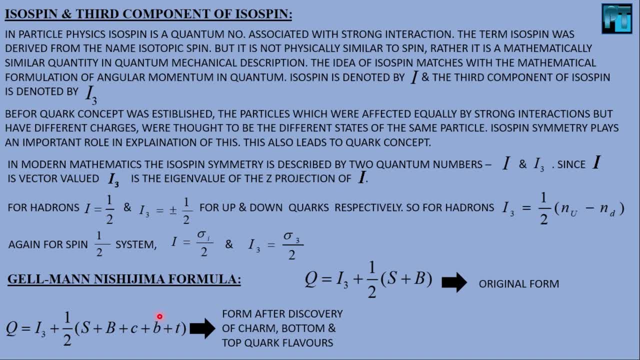 as we know that y is equal to s plus b, or rather accurately, s plus b plus c plus b plus t. So we can modify this relation like y equal to two, q minus i, three, How? Now you have to do the math of your own. 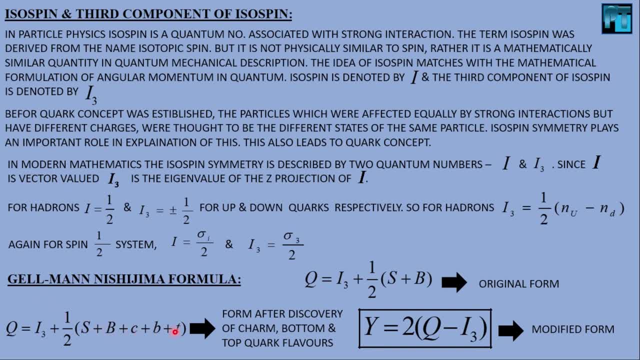 Put s plus b plus c plus b by t, y and rearrange this equation and you will find y is equal to two, q minus i, three. It is the most compact and modified form of Gelman-Nisijima formula In our later lectures. 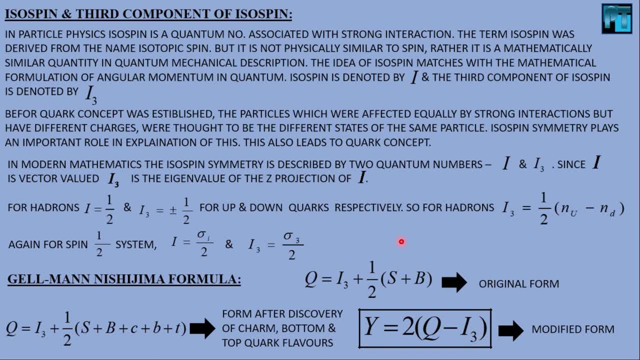 we shall use these quantum numbers and this formula frequently. Okay, guys, So this is the end of our today's discussion. For handwritten notes, please put your email id in the comment box below And if you think that this lecture was helpful for you, 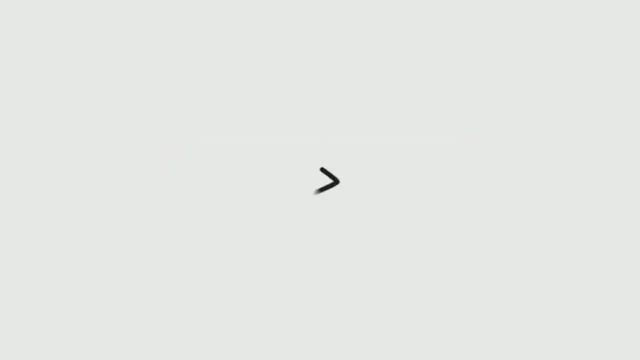 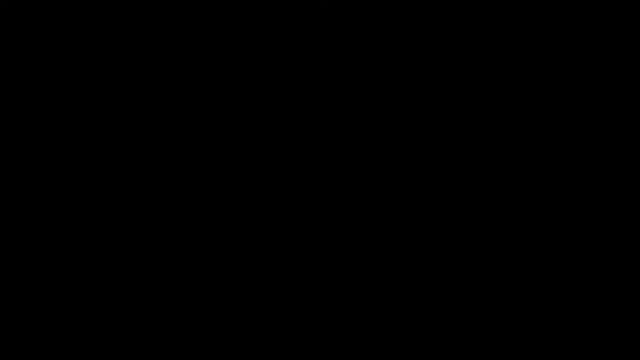